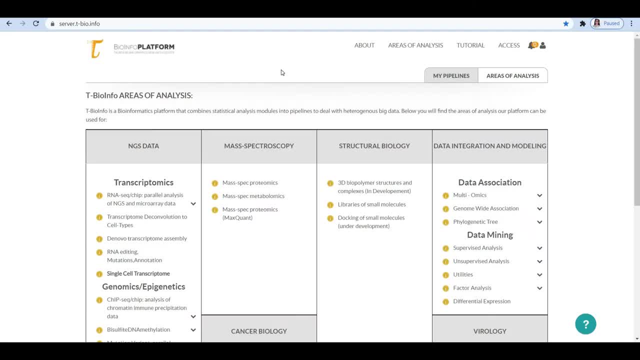 makes it hard to find statistically significant differences. That's why we turn to automated learning, also known as machine learning. This is when we train an algorithm or a machine to perform tasks with data, looking for patterns. Machine learning can be separated in two main categories of methods: unsupervised machine learning and supervised machine learning. 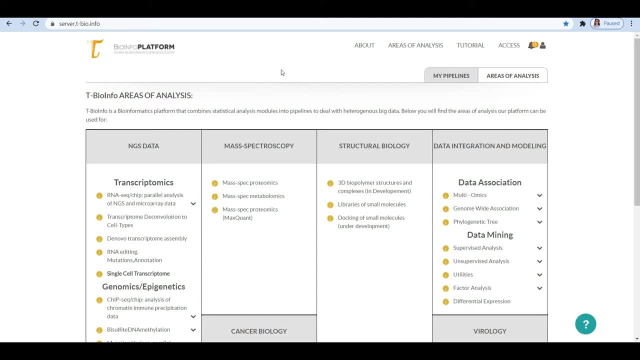 The unsupervised machine learning focuses on detection of patterns in data. The main idea is to separate data into different categories of data. to separate data into different categories, groups or clusters. Often times we can explore the relationship between the defined clusters and known phenotypes to interpret the biological association of. 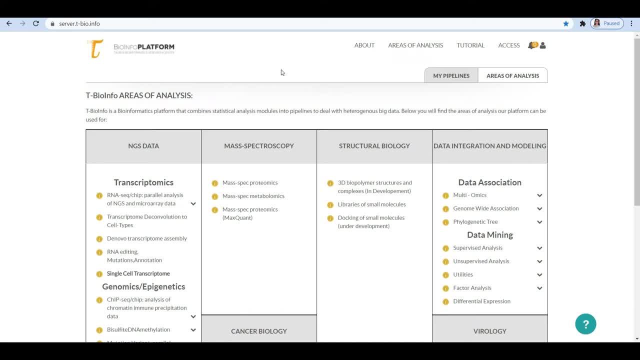 samples in a cluster. Now that the concept is clear, let's try to run several clustering methods and see how they work. To run clustering on tbioinfo platform, you will need to upload the data of expression that we generated from processing the cell line data in the last video. This data can be downloaded. 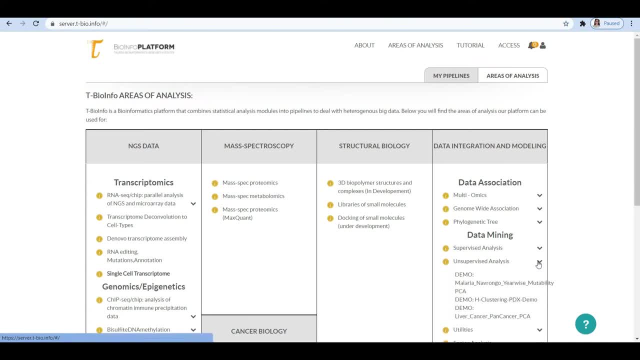 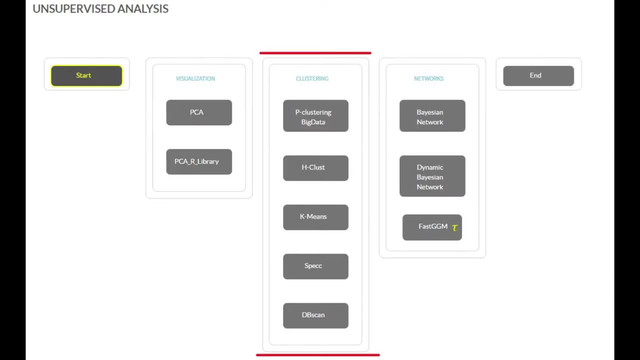 directly from the lesson as well, ie lesson number 13 in the transcriptomics course on the learnomicslogic portal. Clustering methods are located under the data mining section on the tbioinfo server. The tbioinfo platform has several types of clustering methods: P-clustering for 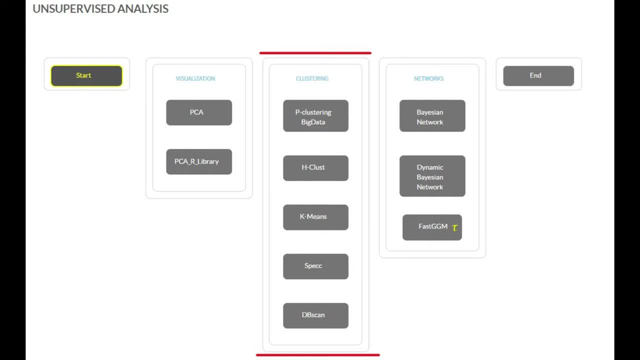 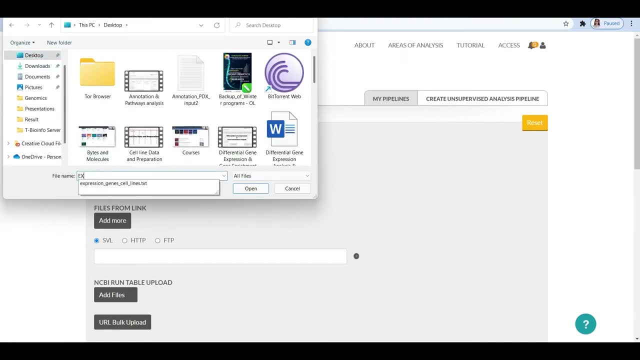 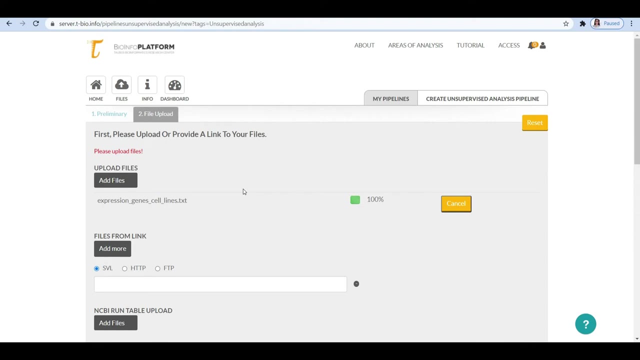 big data, hierarchical clustering, k-means, spec, etc. In this course we will explore hierarchical and k-means clustering, both of which are widely used for analysis of RNA-seq data. Let's run hierarchical clustering to see the analysis output for the breast cancer cell line data, The basic bottom-up. 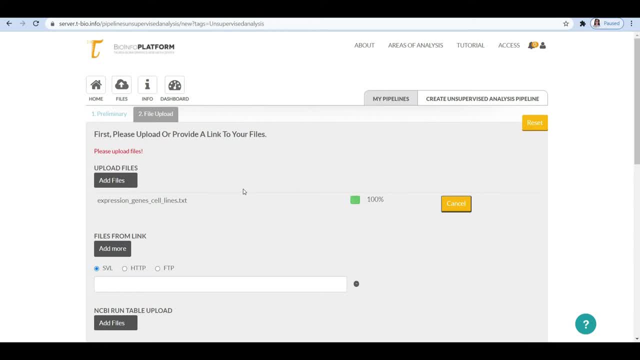 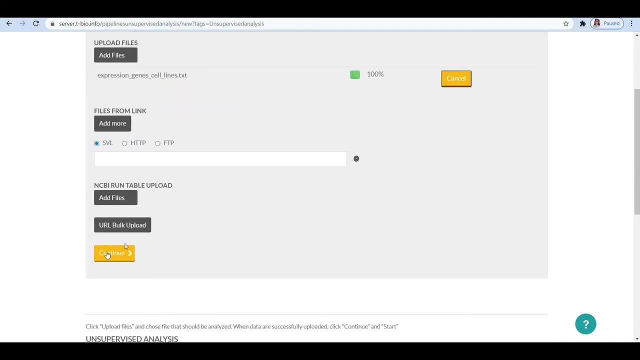 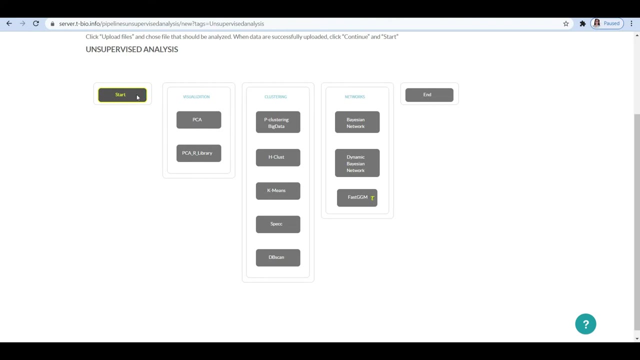 hierarchical clustering algorithm is the edge-cluster module. As in the other methods we have been using in the course, navigate to the data mining unsupervised analysis area, then select File Upload and use the first button to directly upload your file, Start your pipeline and choose edge-cluss from the list of available clustering algorithms.